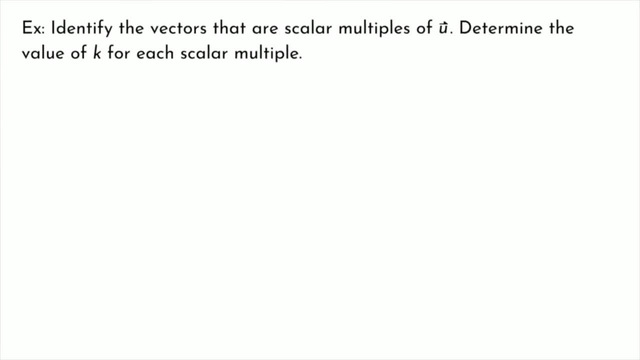 Let's take a look at an example that's going to give you some practice looking at scalar multiples. So this example says: identify the vectors that are scalar multiples of vector u. Determine the value for k for each scalar multiple. All right, so here is our vector u and we're going to bring in a pile of other vectors. 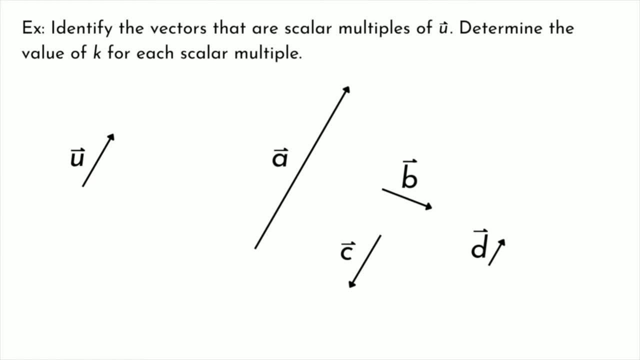 We've got vector a, b, c and d, And our goal is to figure out which of these vectors are scalar multiples of the original vector, vector u. So let's go through these vectors one by one and identify whether or not they are scalar multiples of vector u. We'll start with vector a. 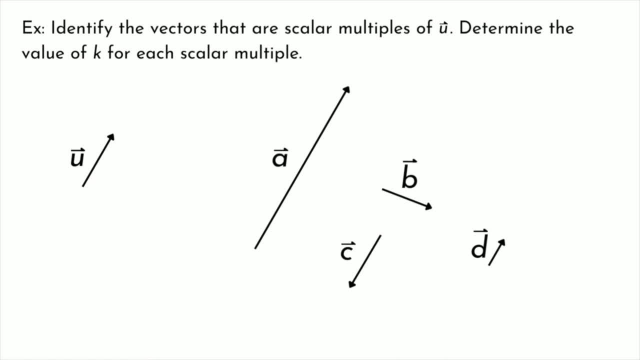 So to find out if a vector is a scalar multiple of another vector, it's helpful to pick up the original vector and sort of place it next to the vector in question, And when we do that we can see that vector u and vector a are parallel. They have the same direction. 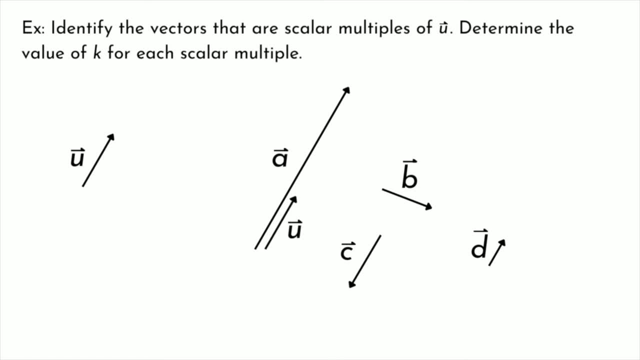 but they don't have the same size. Vector a has a much bigger magnitude than vector u. In fact, if we place three? u's tip to tail, we can see that those three? u vectors will make up one a vector. So we could say that vector a is three times the size of vector u. 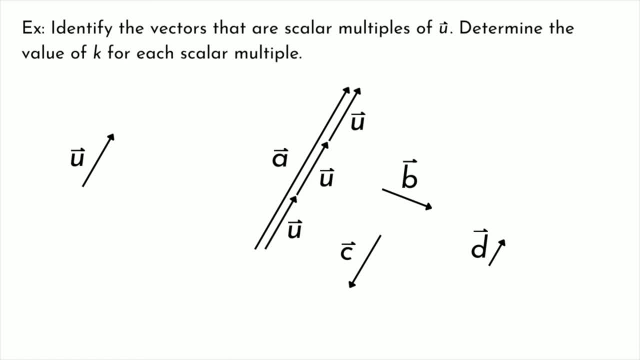 or vector a is a scalar multiple of vector u by a factor of three. We can summarize this by saying: vector a is equal to three times vector u- Right, so here k is equal to three. Let's take a look at vector c. We can see that vector u and vector b are not parallel, And because of this it doesn't. 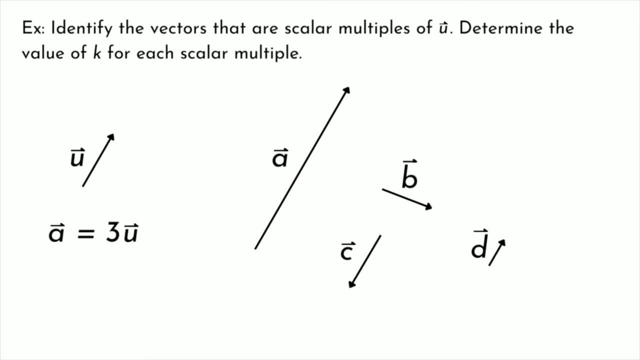 matter what I multiply vector u by, I'll never be able to produce vector b. They might have the same magnitude, but they are not parallel. So we're going to say that these two vectors are not scalar multiples of one another. Taking a look at vector c, we can see that it appears to have the same. 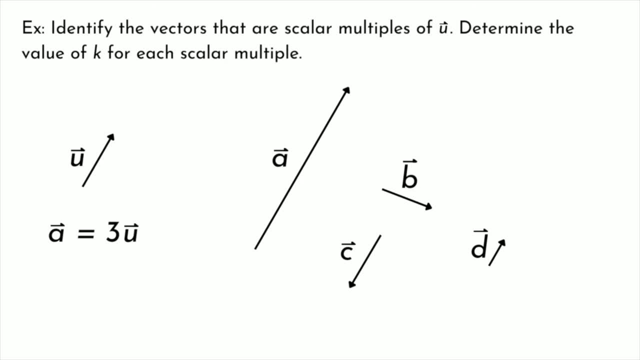 size as vector u, but it's traveling in the other direction. Now that doesn't mean that it can't be a scalar multiple of vector u. We can see that vector c and vector u are parallel vectors. So we can see that vector c and vector u are parallel. Remember that if you want to change the direction. 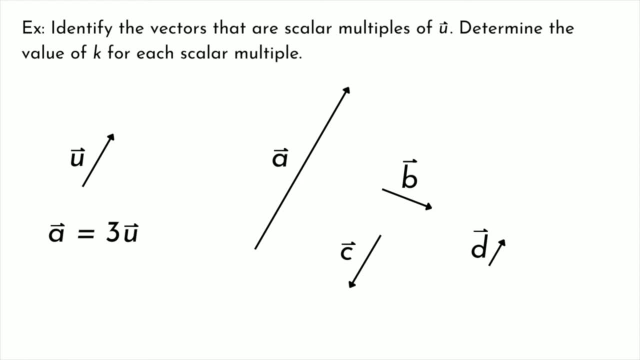 of a vector, we can just multiply it by a negative, Since the magnitudes are the same. in this case, I can take vector u and multiply it by negative one and say that vector c is just equal to negative vector u. So in this case the value of k would be equal to negative one.